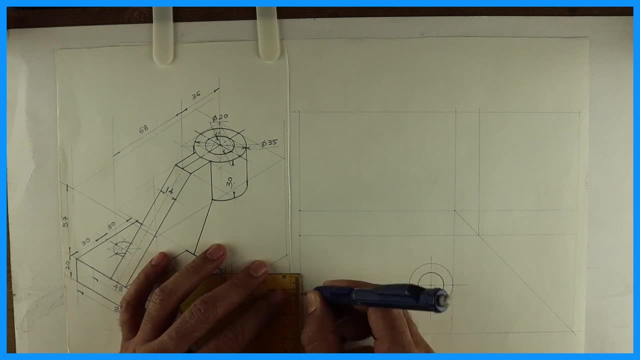 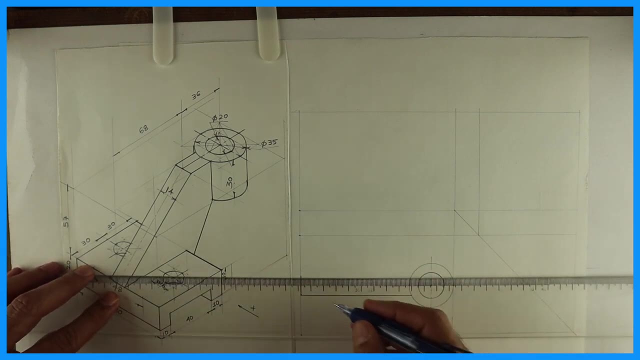 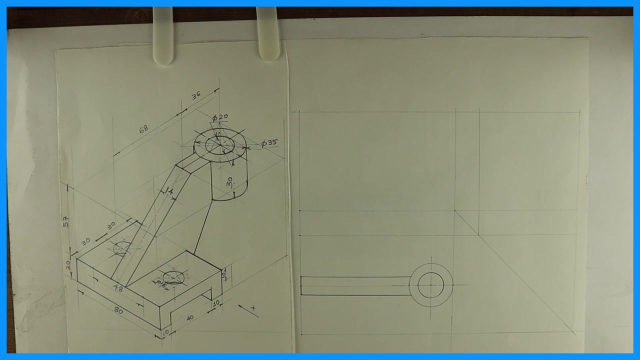 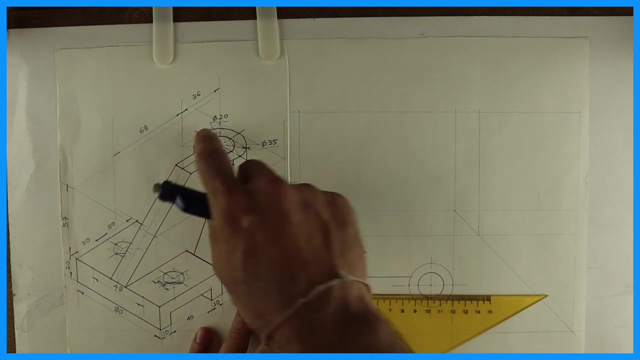 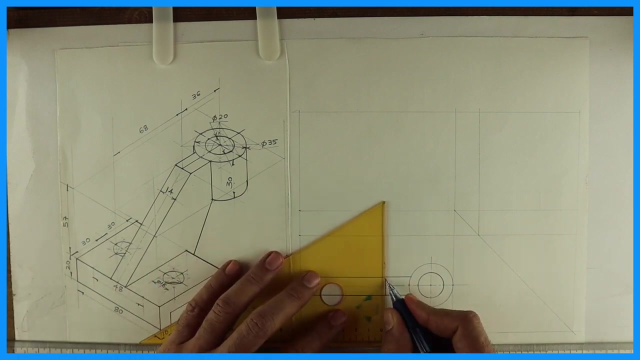 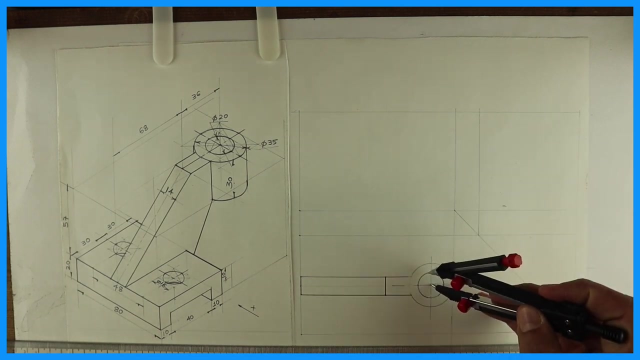 it is 77 on both the sides. If you see that rib, the inclined portion, it is 77 mm on both the sides. So I can take like this: Now I will take 68.. This won't be there In question. also, it won't be there Because it is same surface. 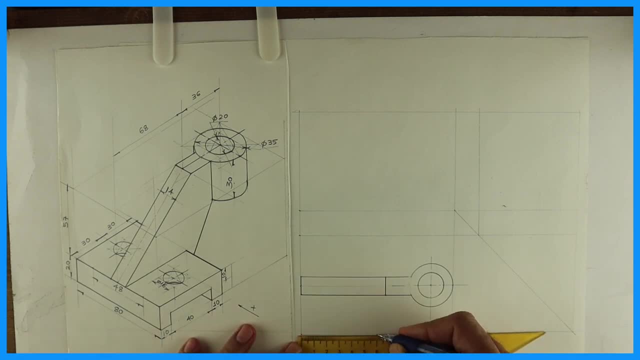 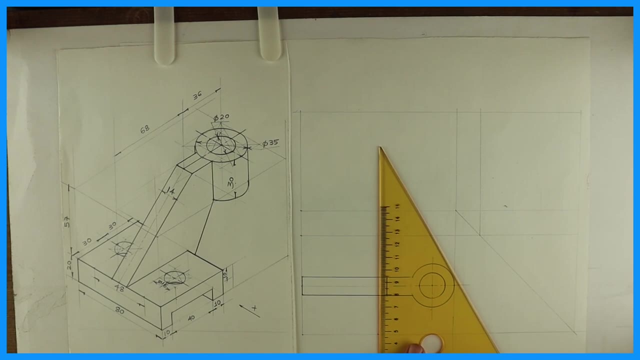 So this is how it will look from top. Now I will take 60 from here. I will draw vertical line. See this portion. So the bottom plate is ready. Now, if you see, over here also there is a dotted line, Because this portion you can't see from. 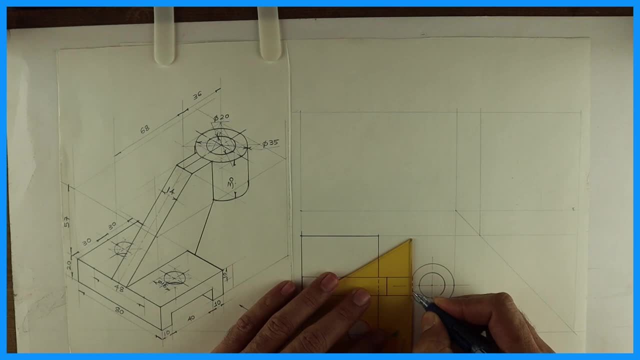 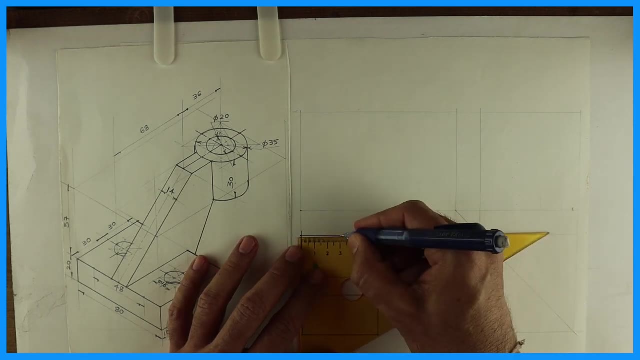 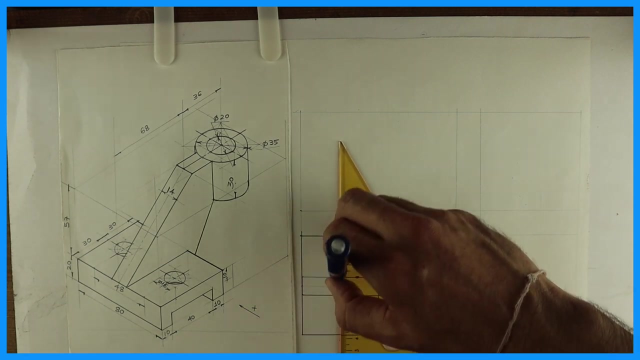 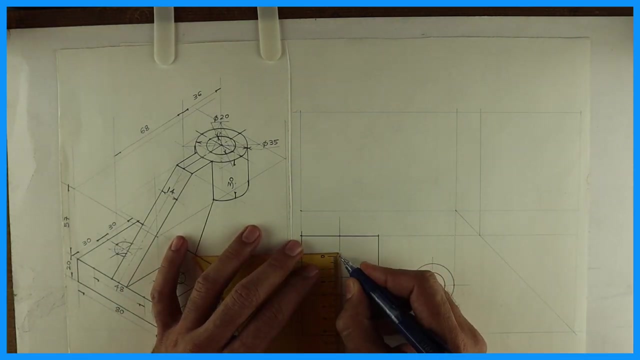 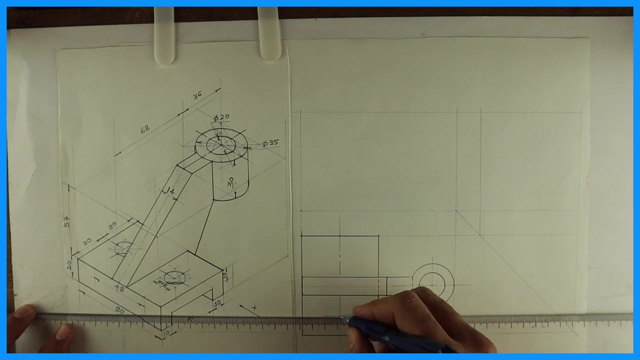 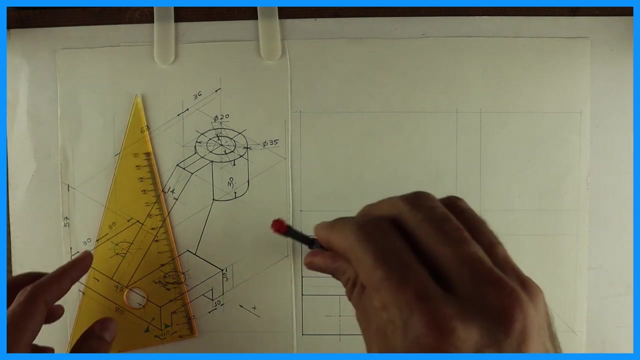 the top. See this, And this part is also dotted. Now there are two circles, So you will take midpoint, Then from center, you take 24, 24.. Then, from center, you take 24, 24.. This will look like a circle. 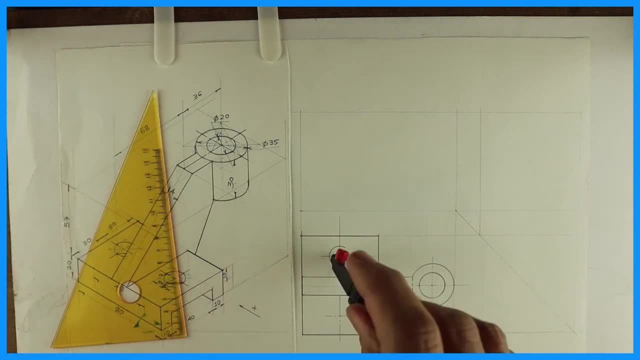 then we will take radius 8. Because diameter is 16. So you take radius 8. And you can draw circle. All should be same: Superb, Very bri, very big circle. You can draw whatever you want to call circle here. 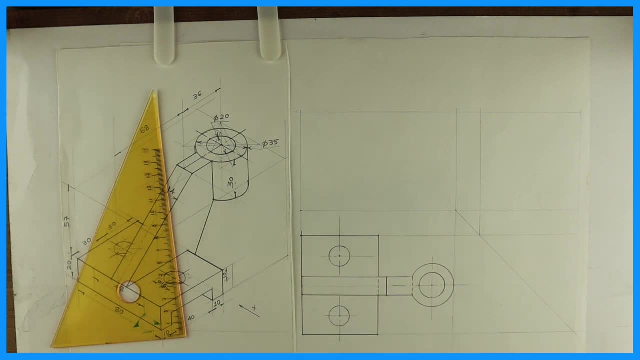 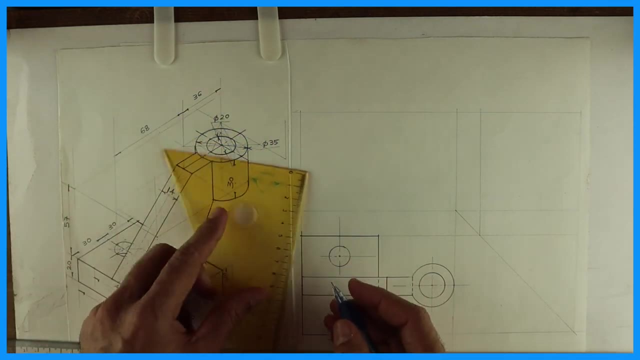 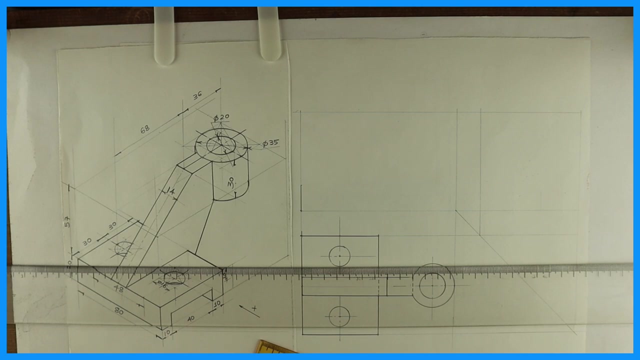 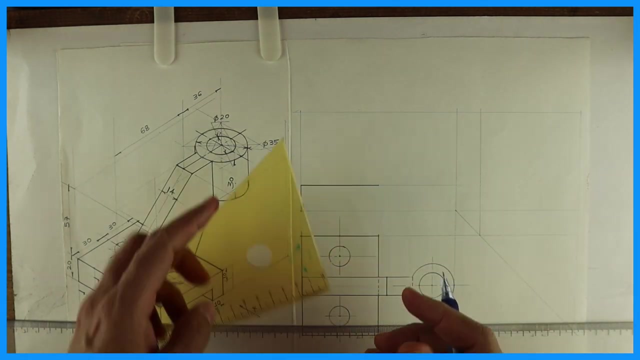 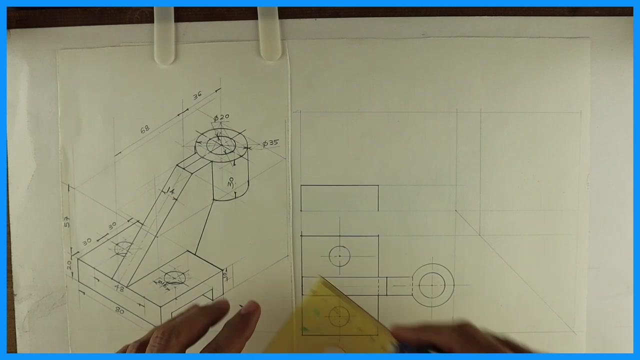 So you can draw circle as many as you want. After that we will draw this part. see in front view. this height is 20, so we are drawing lower block in front view: 20 by 60.. This is 10,, 40,, 10.. 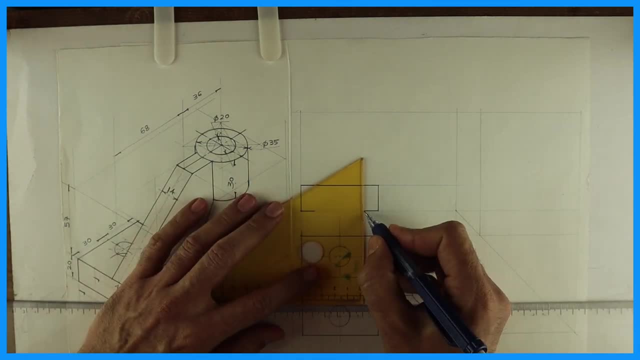 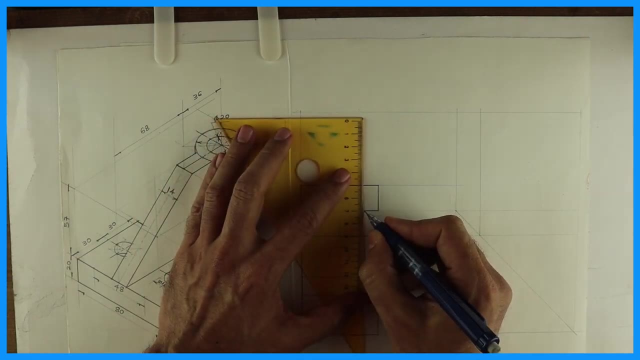 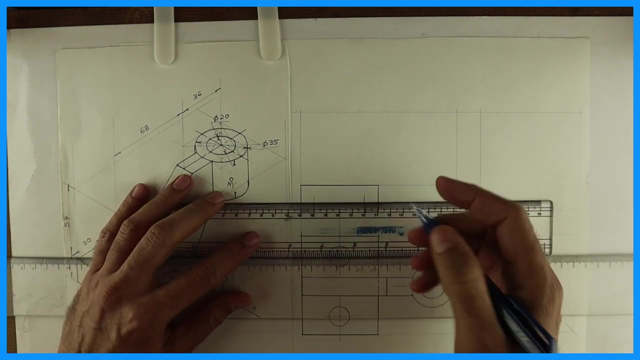 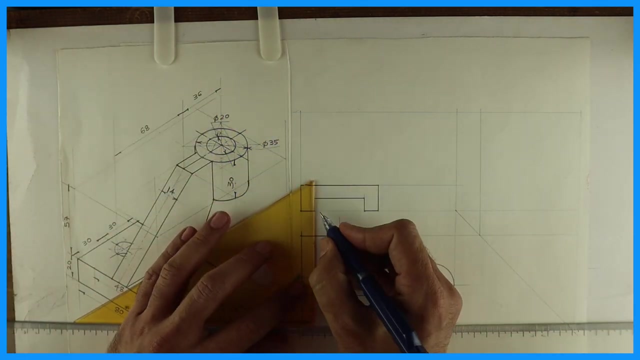 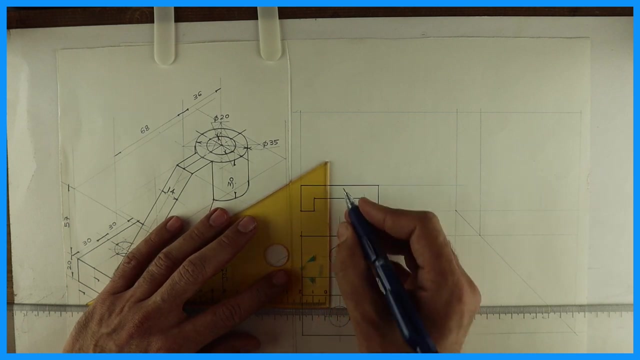 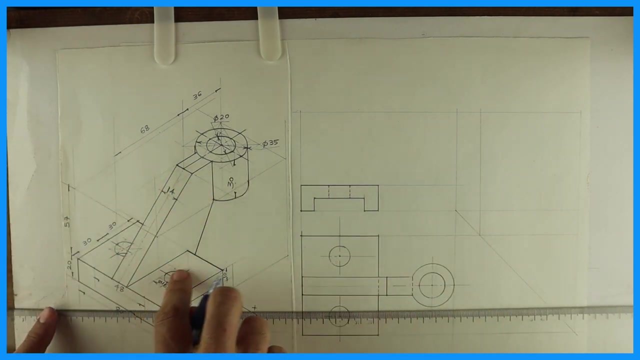 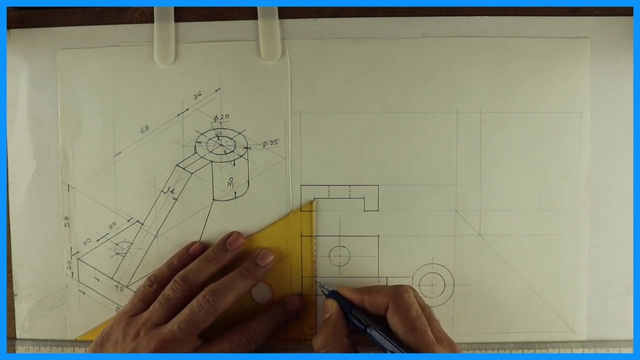 Ok, This height is 10.. This height is 10.. Now we will draw dotted line for this circle: extreme L, extreme left and right, So LRTB concept, so L and R, both the circles. And we will draw dotted line for this in top view because this is through and through. 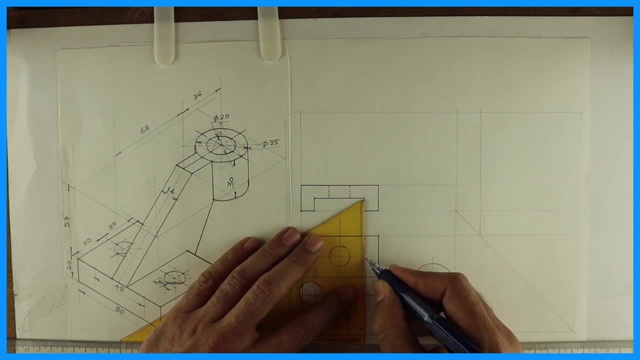 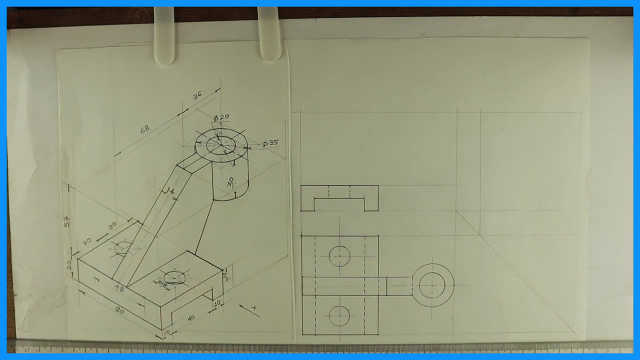 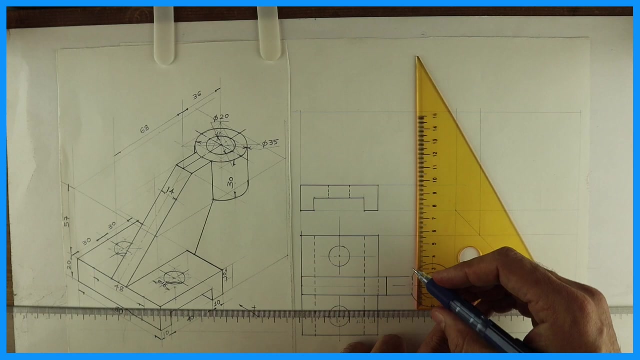 See this. So we will have two dotted lines. Ok, Ok, Ok, Ok, Ok, Ok. Now we will hide this circle. this height is 30.. This circle is in right of our circle. Ok, Ok, Ok. 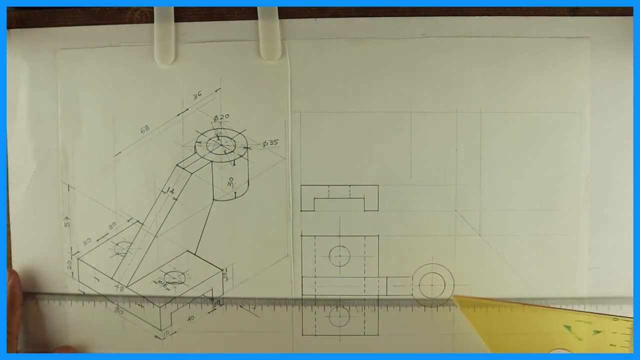 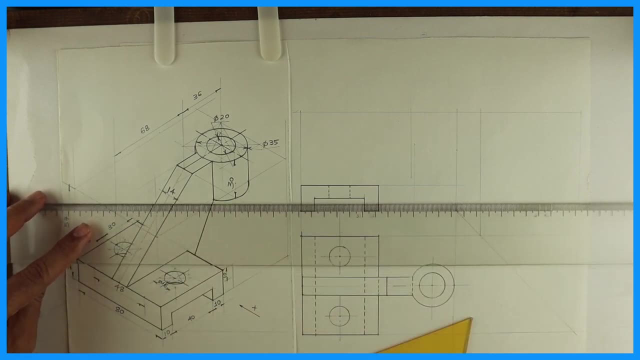 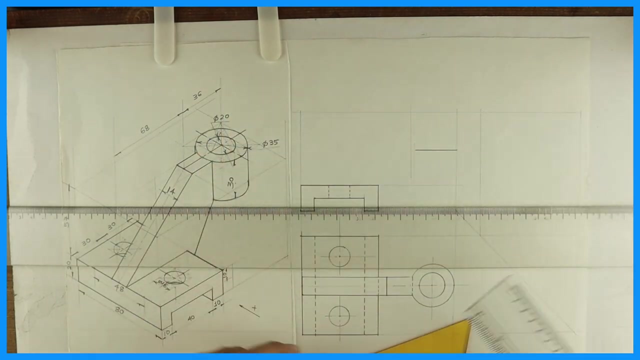 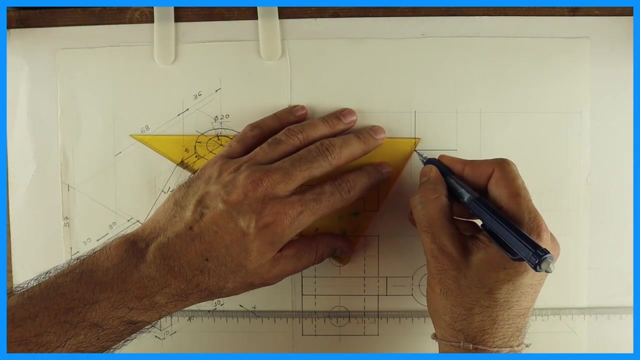 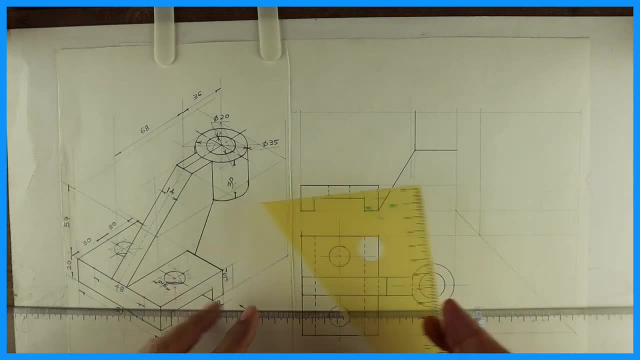 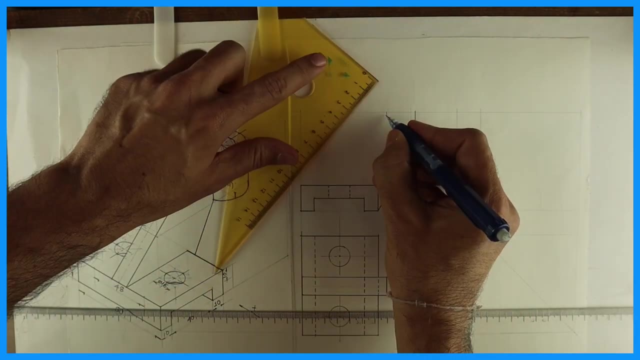 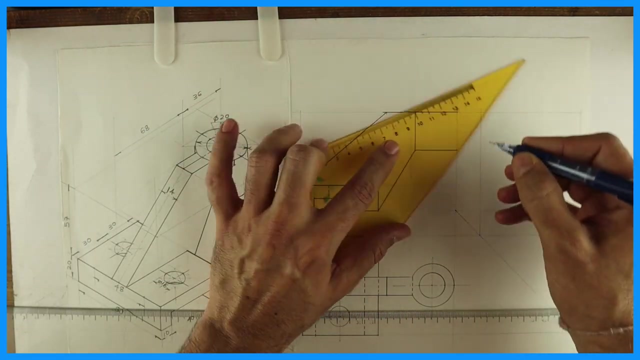 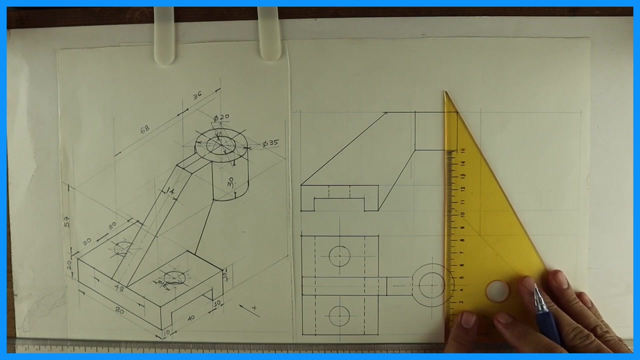 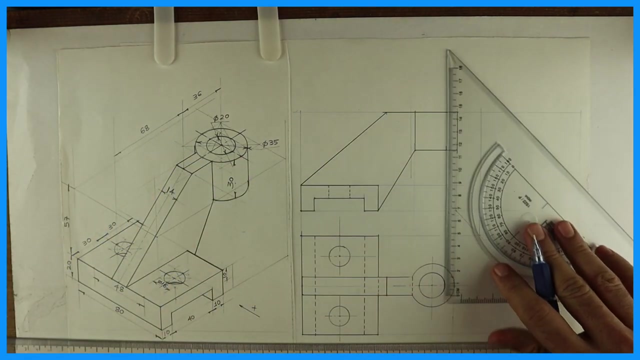 and this slope is also there from center, how much it is away? 36, so that I can take projection from top view also. so I'll get that point. from that point to this point I can join so that inclined portion is done. after that, from here we can draw dotted line. 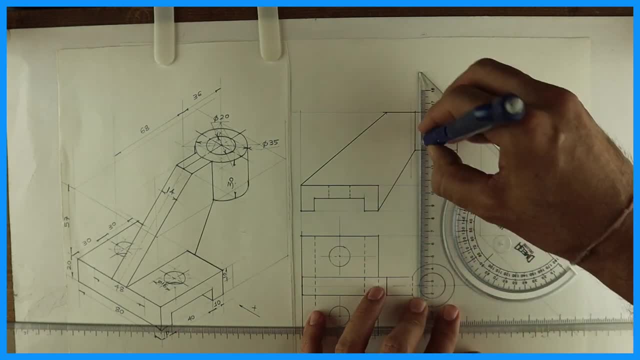 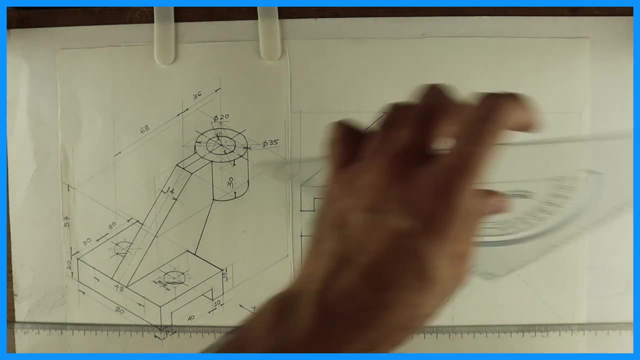 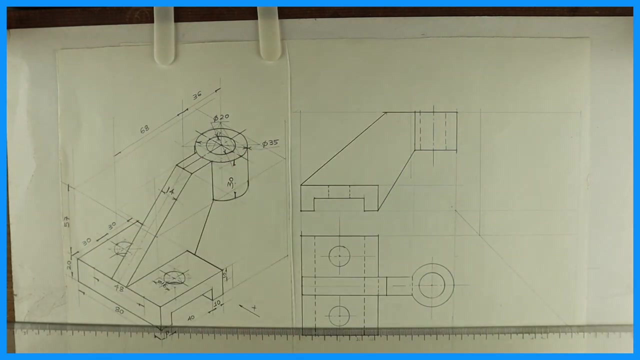 this is extreme right point of the circle and we'll draw extreme left point. always remember: in front view you will have LR. In side view you will have tb. extreme top and bottom point, We will have center line for this. so we are done with front view as well. 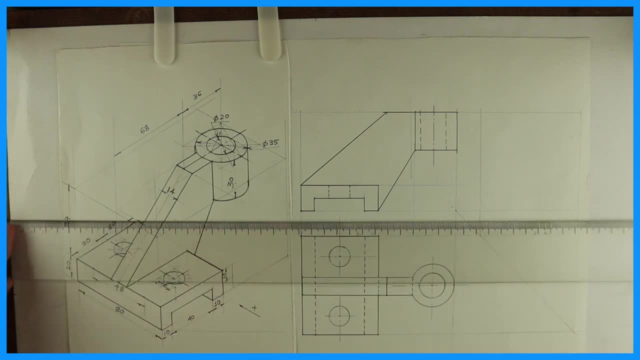 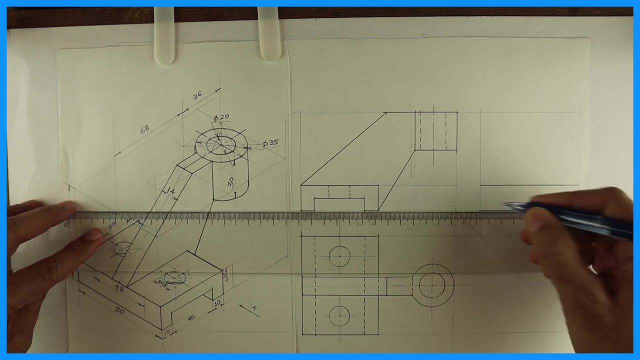 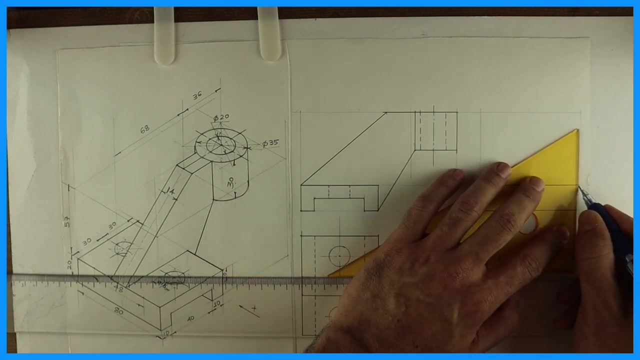 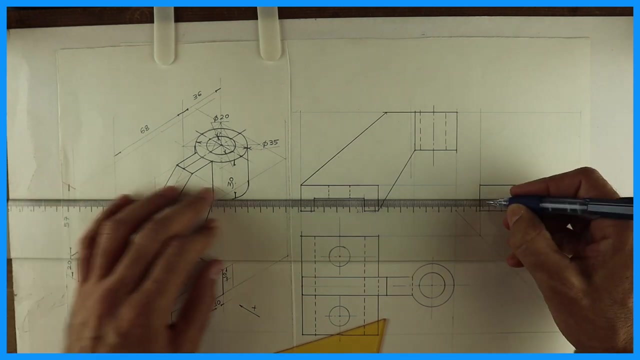 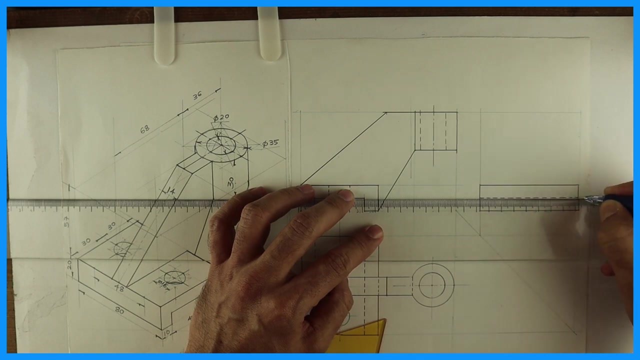 Now we will try side view. side view: you will see this part rectangle. so we will draw that rectangle first. that 20 by 80, we will draw that first. we will draw vertical line. see, then it is going through and through. so from here this will be through and through. 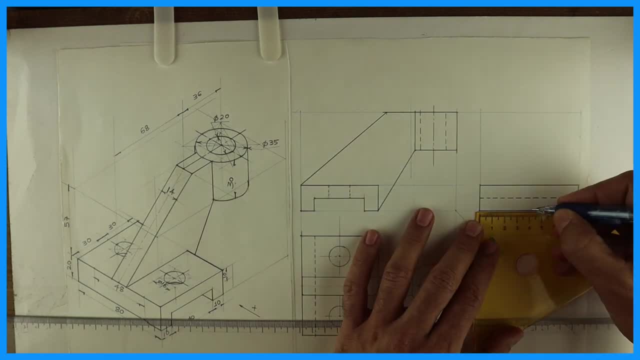 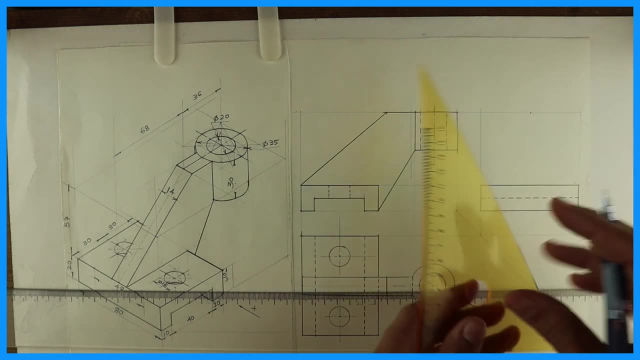 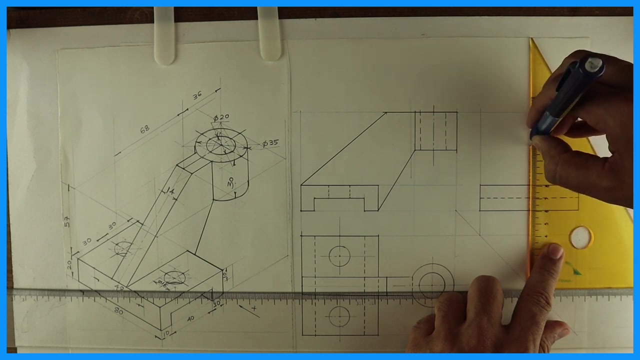 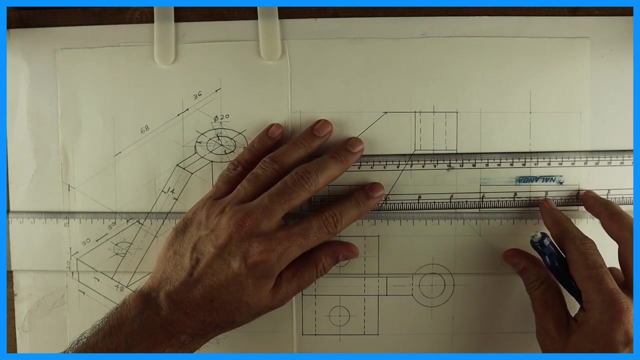 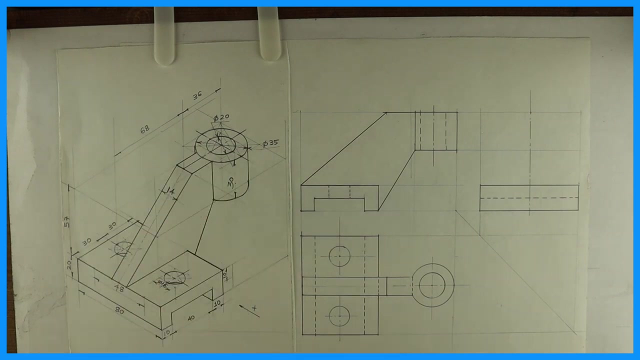 After that, this slope, so it will be rectangle, this is 40,. you take midpoint 40,. this is 40,, this is 40, then again rectangle for the circle that is diameter 35, so from center I can mark 17.5,, 17.5, or I can take lines from top. 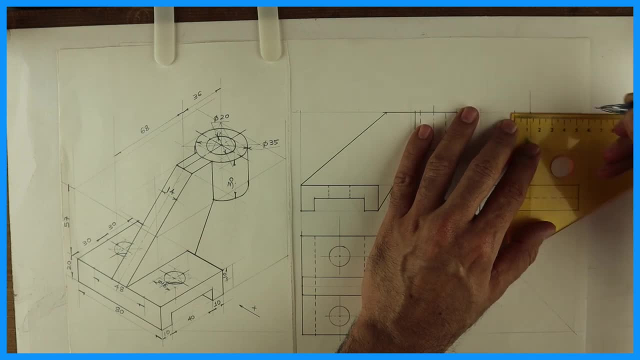 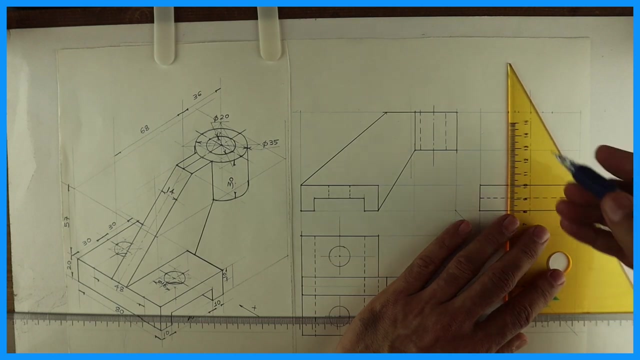 So this is the circle. You can see, here it is 20 and I can take lines from top and top. so here I am taking right sides. so we will now take 1,, 2,, 3, 4,. 1,, 2,, 3,, 4,, 5,, 6,, 7,, 8,, 9,, 10,, 11 and 11, and 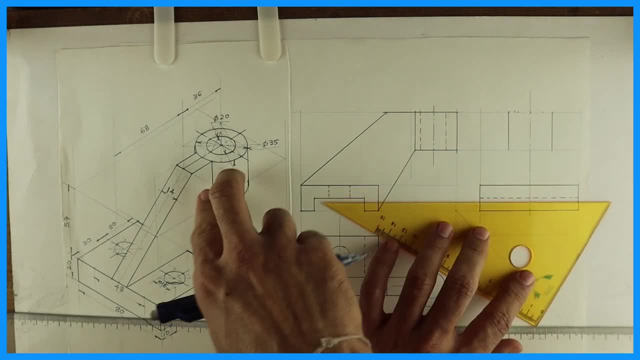 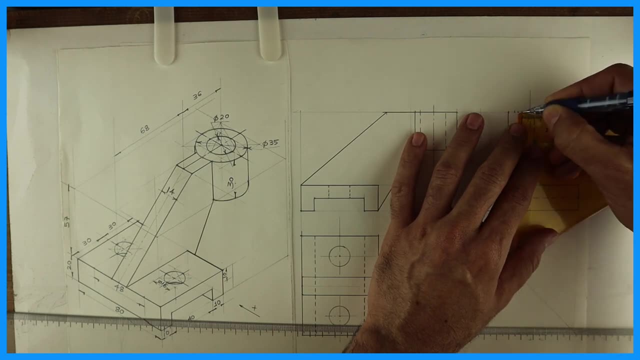 10,, 11,, 12 and 13,, 13,, 14,, 14,, 15,, 17,, 18,, 19,, 19,, 20,, 21.. So that is the horizontal. You can see the distance here. 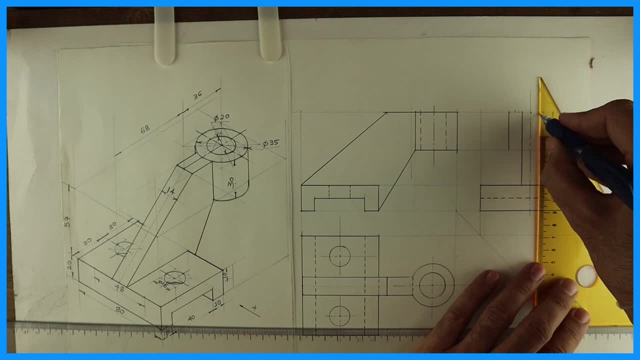 So that is the same as the vertical. So that is the distance. here I have the días. this is the distance. now we have a left and this is the right. this- This is rectangle inclined portion- will be appearing as a rectangle in side view. this: 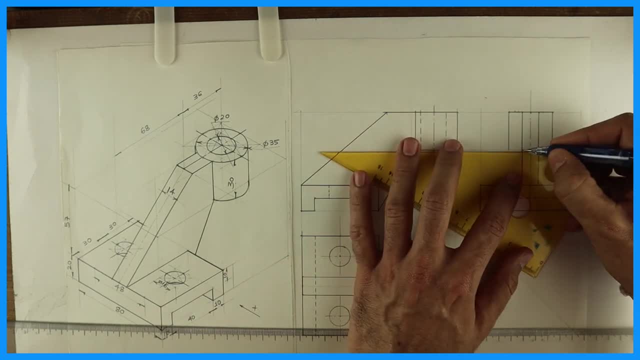 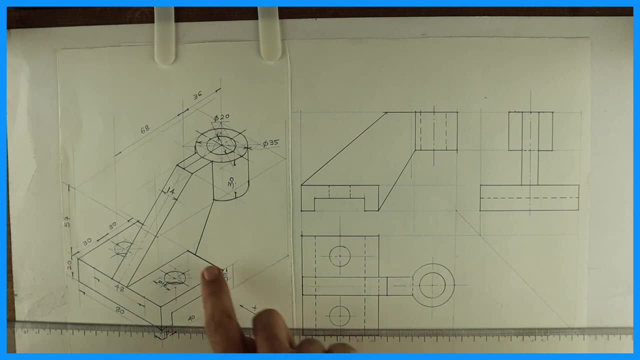 will be dark. So we are done with side view. also, only dotted lines are remaining. This will be dotted because you can't see the behind portion. Then this circle, this part, is also going through and through. see this, this part. 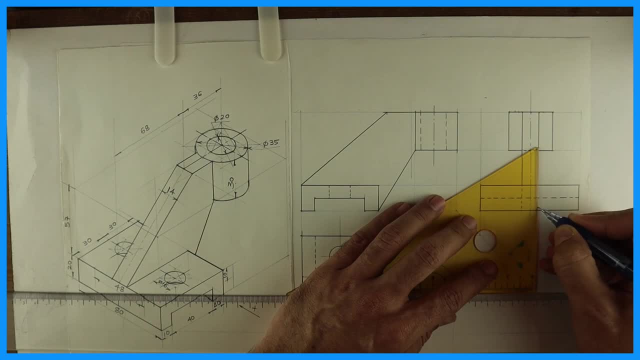 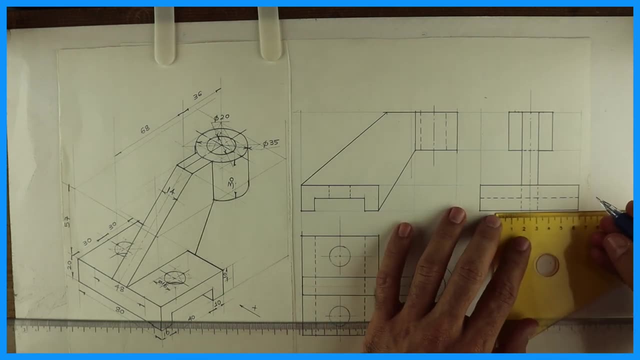 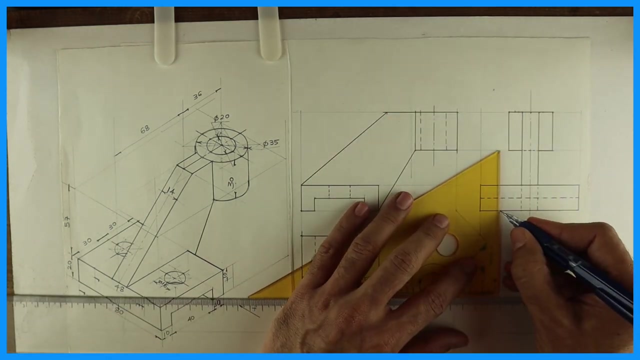 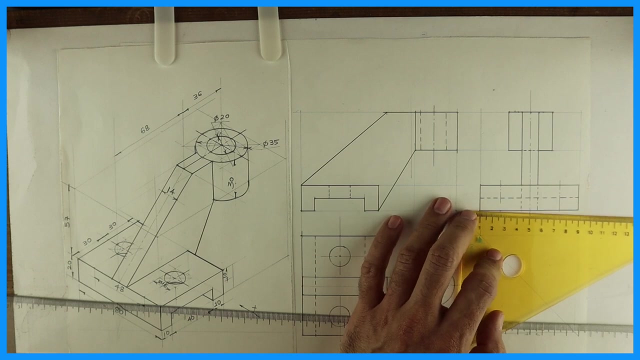 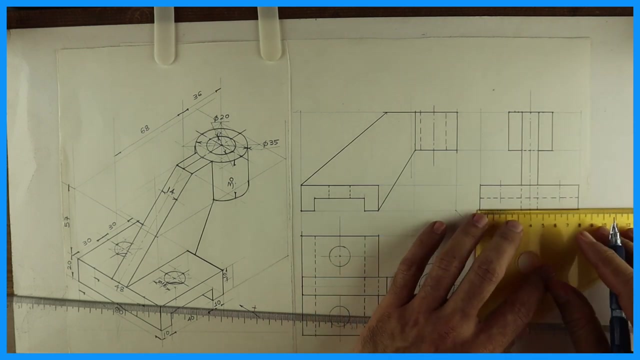 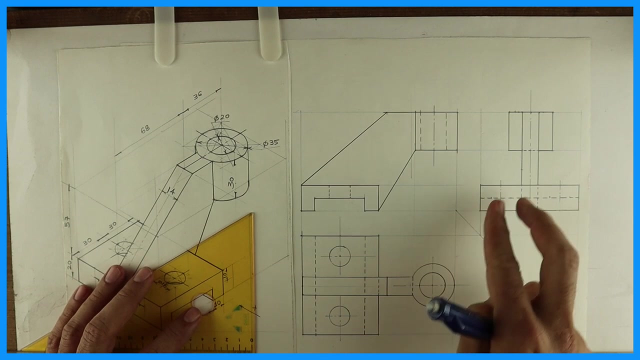 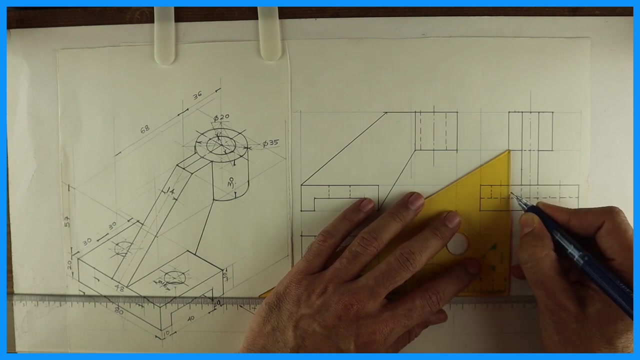 So this is dotted. This is also dotted. Now we need to draw dotted line for the circle This, radius 8, diameter 16. So that also we can mark. You can take 24, 24.. See this over here you can draw dotted line in side view. that is TB, extreme top and 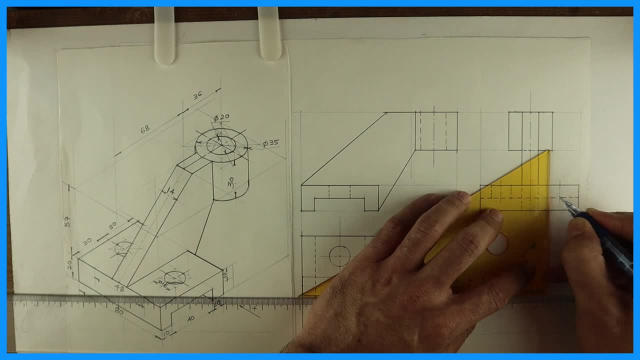 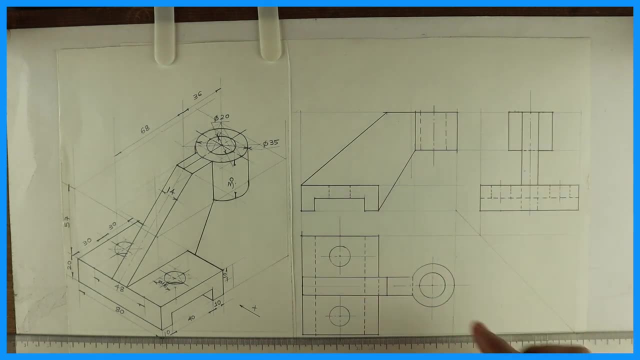 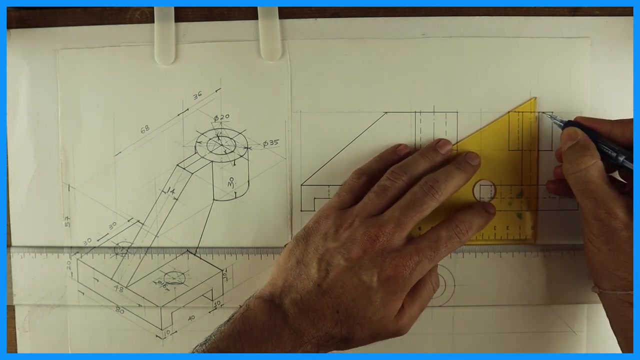 bottom point. You can take it from top view also, or you can take from center line 88. After that, diameter 28.. Okay, Dimeter 20, that also we can draw. So we are done with side view also. So we have done front view, top view, side view of the sum in first angle method.